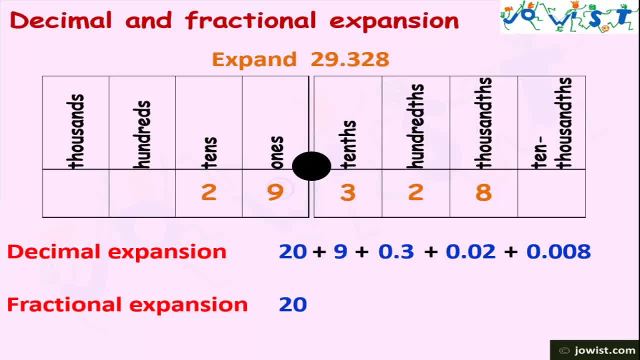 we will write 20 plus we have 9 ones. so we will write 9 here. These are the whole number part Plus we have 3 tenths. so we will write 3 upon 10 plus we have 2 hundredths. so we: 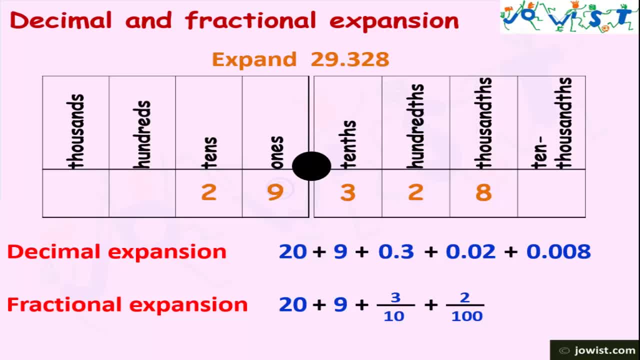 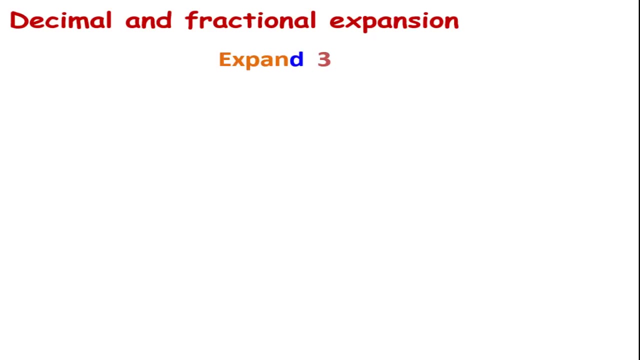 will write 2 upon 100.. Plus we have 8 thousandth, so we will add 8 upon 1000.. It is equal to 8 upon 1000.. One more example will help us to understand it better. Let's expand the number: 371.1452.. 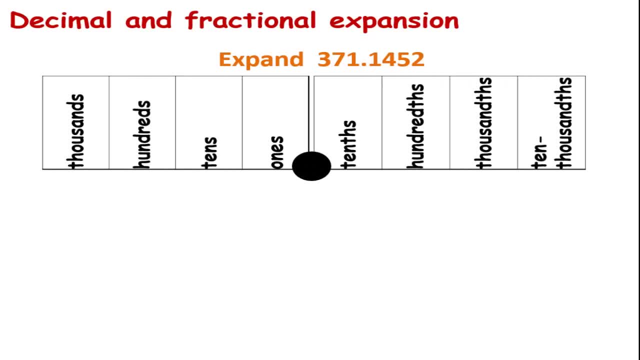 Let's expand the number with the help of place value chart. We will write the number as shown. It means the number before the decimal point is written left to the decimal point, that is, 371, and numbers after the decimal point is written after decimal point, like we have. 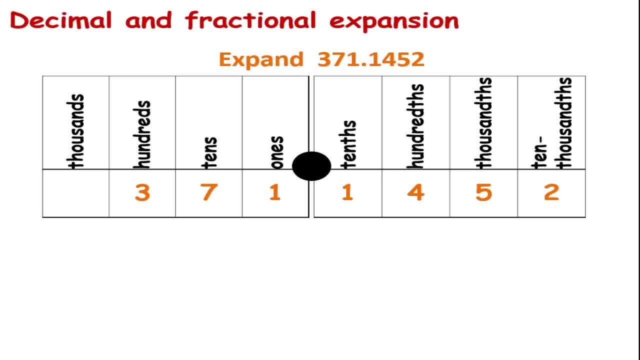 done for the number 1452.. Now look at the decimal expansion of this number. We have 352.. so we will write 300 plus. we have 7 tenths, so we will write 70.. We have 1 ones, so we will write plus 1.. Now we have 1 tenths, so we will write plus 0.1.. As we have 4 hundredths. 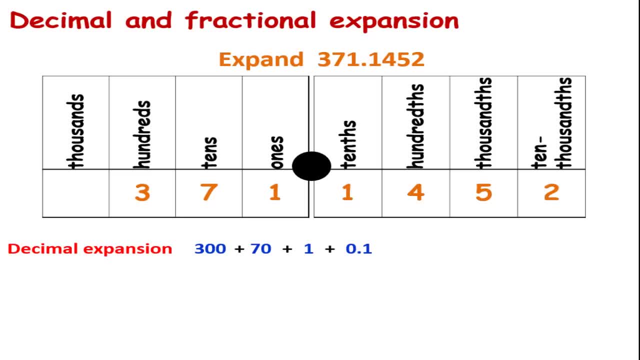 so we will write plus 0.04.. We have 5 thousandth, hence we will write plus 0.005. and we have 10 thousandth position and in the 10 thousandth position we have 2 plus 0.005.. So we will.